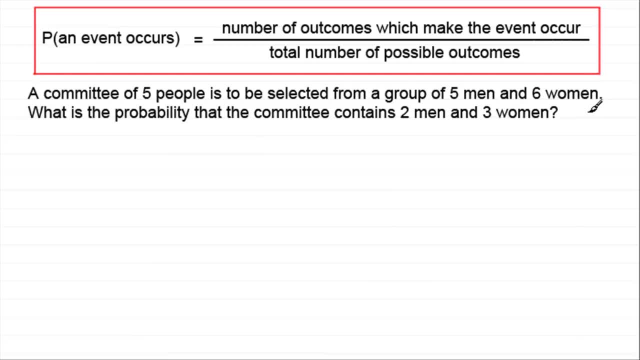 that the committee contains two men and three women. So, in order to do this, what I need to do is work out each of these values in this formula. I'm going to start with the denominator. I always think that's the easiest part to start with in questions like this. Total number of possible. 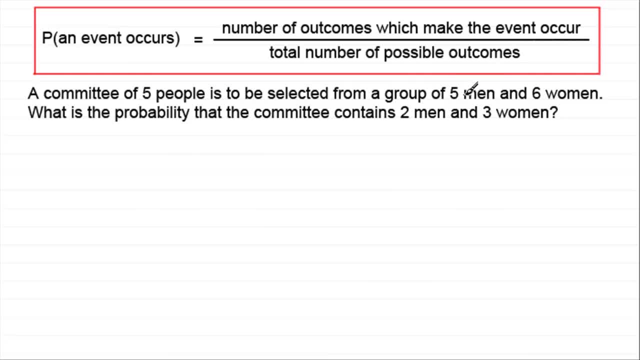 outcomes For this question. it'll be the total number of committees that we can form, having five people in. So to do this as well, what I'll do is have some dashes here to represent the order in my formula. So, when it comes to looking at how many ways we can form a committee from, 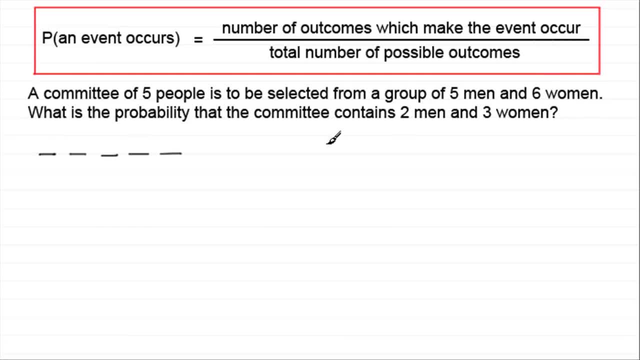 eleven people, that's the five and the six. how many different ways is that going to be? Let's just put the number of committees here that we can form. Now for something like this, we've also got to determine whether we've got a permutation or a combination. Permutation order matters Combination. 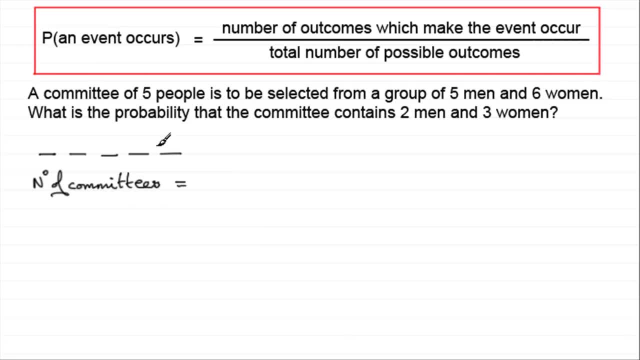 Well, this is going to be a combination. It's a selection of people. Order doesn't matter. So what we've got is we can place 11 people in, or we've got a choice of 11 people for this first slot, So that's going to be 11.. Once we've chosen one of those 11 people, we're now down to 10 to fill the next space. 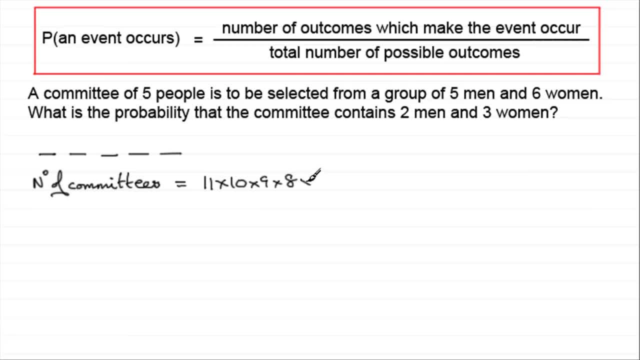 And then 9,, and then 8, and then 7.. But do you remember, this gives us a permutation, The number of different ways that we could fill these slots if it was an arrangement. But within those values there, within those arrangements, remember that these 5 people can arrange themselves within themselves. 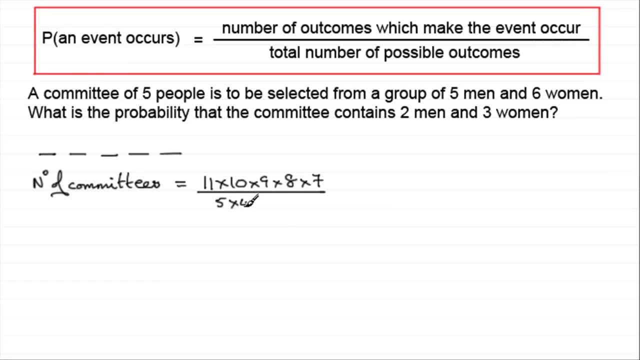 5 factorial ways. So we need to divide this by 5 by 4.. By 3, by 2, by 1.. Now you could have done this by using the combinations formula, Because it's a simple based problem. We've got no repetition or anything like that. 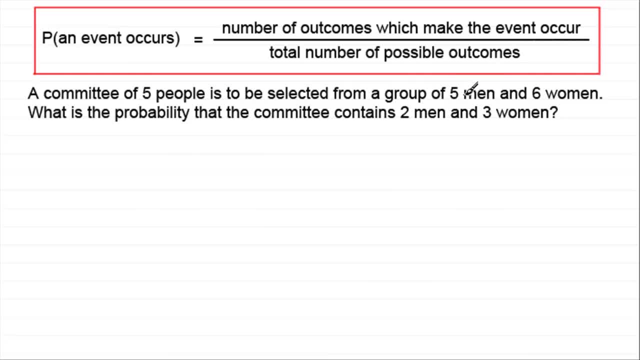 outcomes For this question. it'll be the total number of committees that we can form, having five people in. So, to do this as well, what I'll do is have some dashes here to represent the number of possible outcomes. So, when it comes to looking at how many ways we can form a committee, 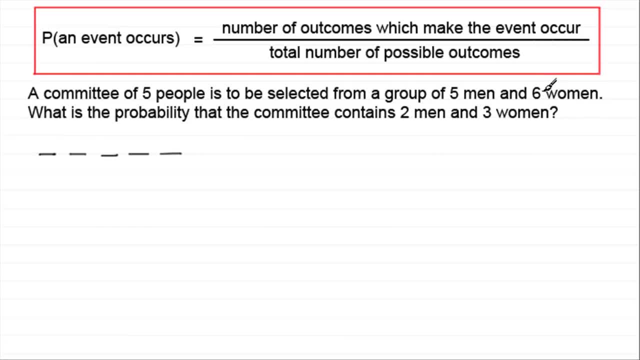 from 11 people, that's the five and the six. How many different ways is that going to be? Well, let's just put the number of committees here that we can form. Now for something like this, we've also got to determine whether we've got a permutation or combination. Permutation order matters combination. 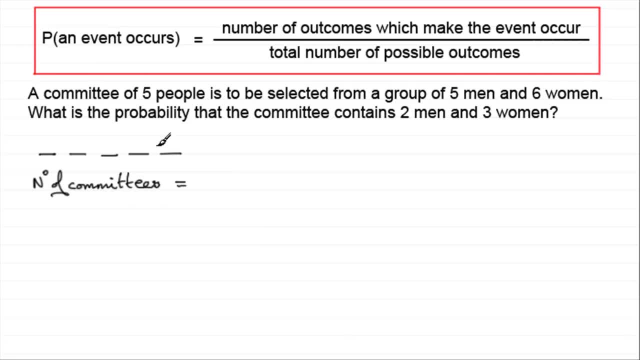 order doesn't matter. Well, this is going to be a combination, It's a selection of people. Order doesn't matter. So what we've got is we can place 11 people in. well, we've got a choice of 11 people for this first slot, So that's going to be 11.. Once we've chosen one of those 11 people, we're 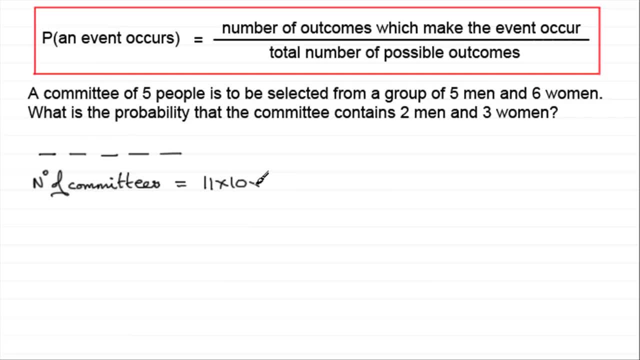 now down to 10 to fill the next space, And then 9, and then 8, and then 7.. But do you think that's going to be a permutation? Yes, it is a permutation. So remember, this gives us a permutation. The. 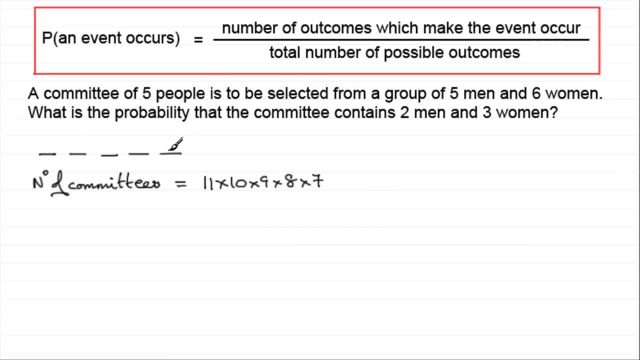 number of different ways that we could fill these slots if it was an arrangement, But within those values there, within those arrangements, remember that these five people can arrange themselves within themselves five factorial ways. So we need to divide this by 5, by 4, by 3, by 2, by 1.. Now 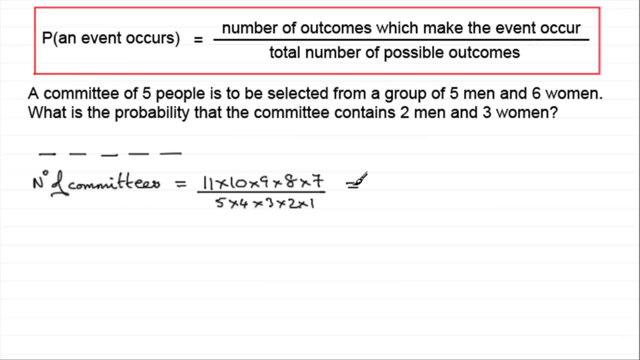 we need to divide this by using the combinations formula, because it's a simple based problem. We've got no repetition or anything like that, So you could have said: well, OK, I've got 11 people and I want to choose just 5 people. If you were to work that out, it's exactly this formula here. 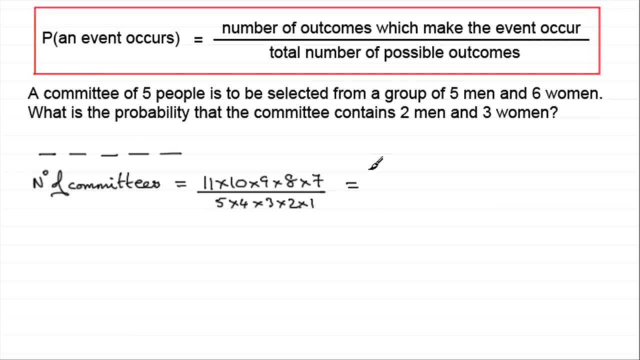 So you could have said: well, ok, I've got 11 people And I want to choose just 5 people. If you were to work that out, it's exactly this formula here, And what it comes to is 162.. 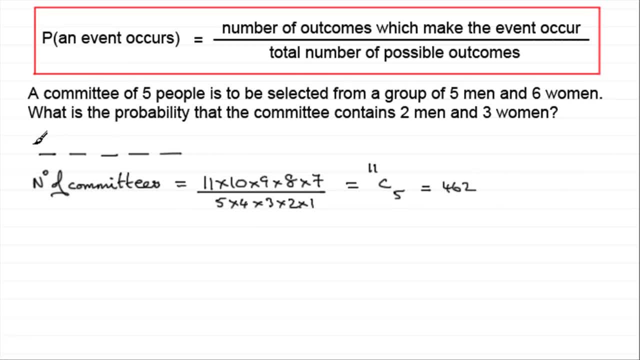 Now we need to look at the special case now. How many committees consist of 2 men and 3 women? So we'll just put down here the number with. We'll put it in brief: ok, 2 men and 3 women. 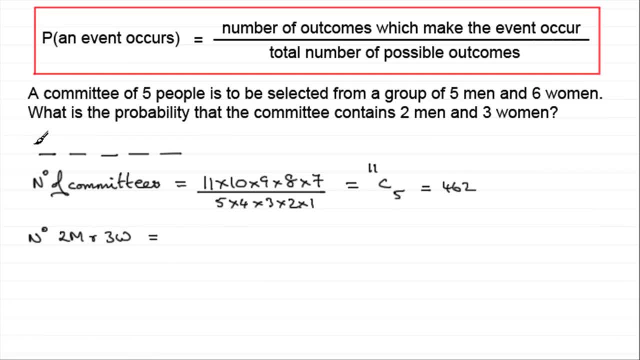 How many would that be? Well, let's just put man 1, man 2 in here, if you like, And then Woman 1, woman 2, woman 3.. We're not interested in the order here, though, So what about the 2 men? 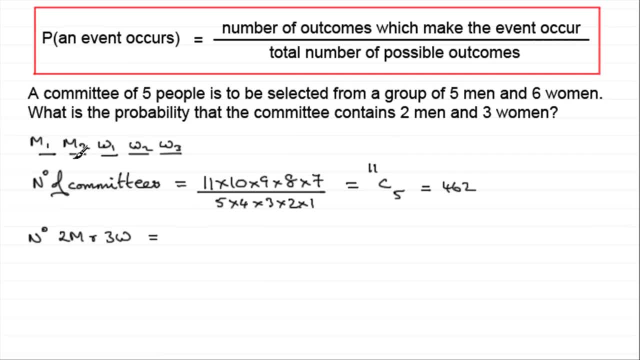 How many ways can we select 2 men to put in these slots here? Well, we've got from 5 men. we can fill that first slot 5 ways. This slot can be now any of 4 ways, So 20 ways that we've got of essentially. 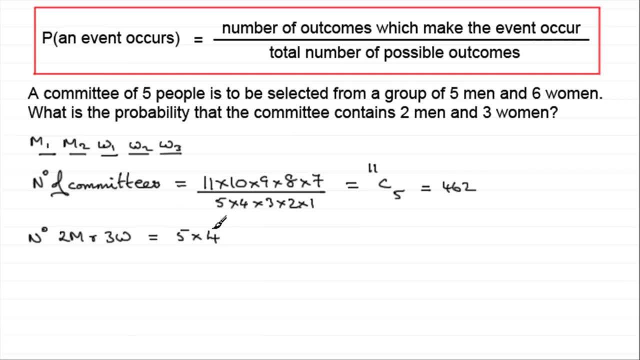 Taking 2 men And arranging them. Remember, this gives the arrangements, But within any of those arrangements the 2 men can rearrange themselves amongst themselves. 2 factorial ways: 2 by 1. So that's the men taken care of. 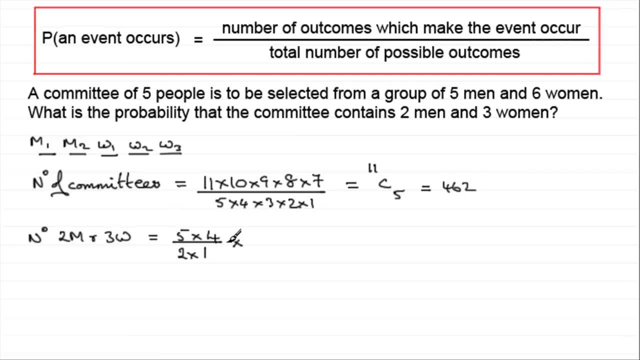 Now, because it's in the same problem, we need to times by how many ways we can put the women in here, And so for the first woman out of 6, there'll be 6 ways. Then for the next one, there'll be 5 ways. 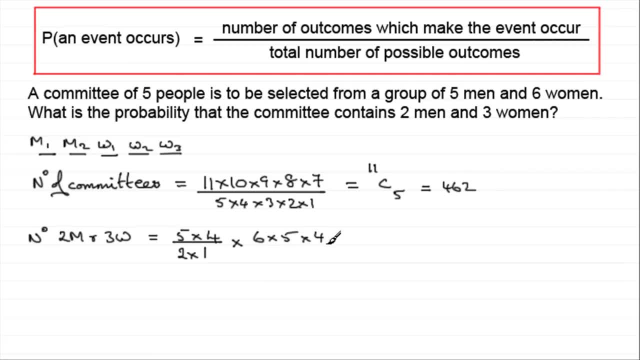 And then for the next one, 4 ways. But this would be the number of arrangements of the women. We're not interested in arrangements, Just a selection Order doesn't matter. So within these 3 women, the 3 women can rearrange themselves amongst themselves. 3 factorial ways: 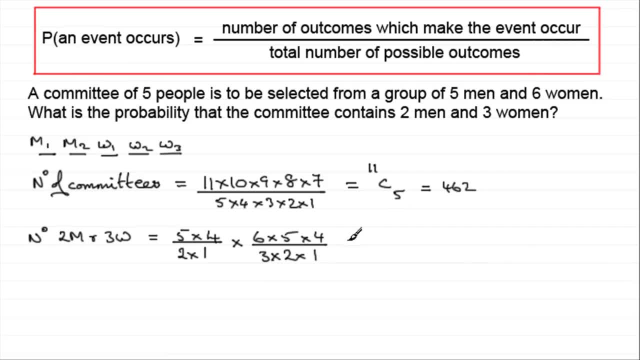 3 by 2 by 1.. And again, you could have done this Through using this, Using combinations, formally, Because what you could have said for the men is that from 5 men choose just 2. And for the women, 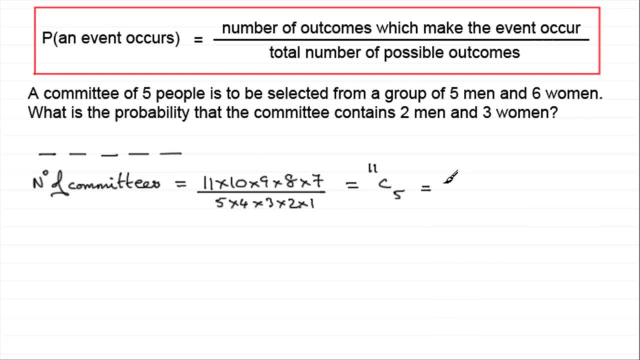 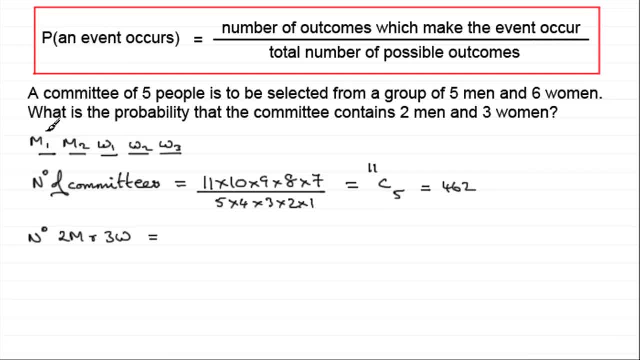 order here, though. So what about the 2 men? How many ways can we select 2 men to put in these slots here? Well, we've got from 5 men. we can fill that first slot 5 ways. This slot can be now. 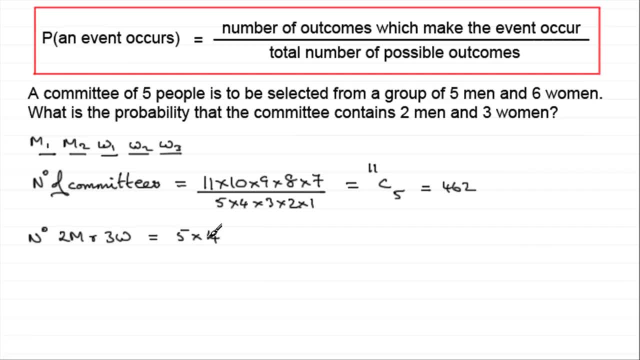 any of 4 ways. So 20 ways that we've got of essentially taking 2 men and arranging them. Remember, this gives the arrangements, but within any of those arrangements the two men can rearrange themselves amongst themselves. two factorial ways: two by one. 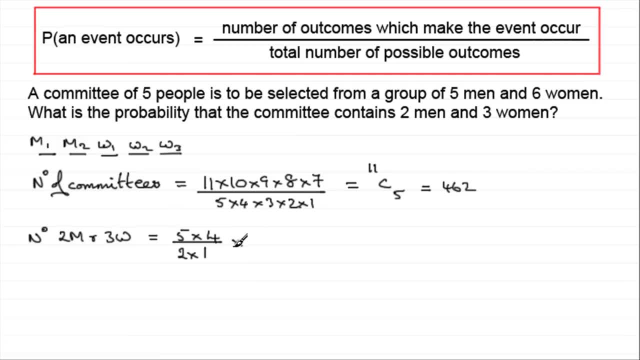 So that's the men taken care of. Now, because it's in the same problem, we need to times by how many ways we can put the women in here, And so for the first woman out of six, there will be six ways, Then for the next one there will be five ways, and then for the next one, four ways. 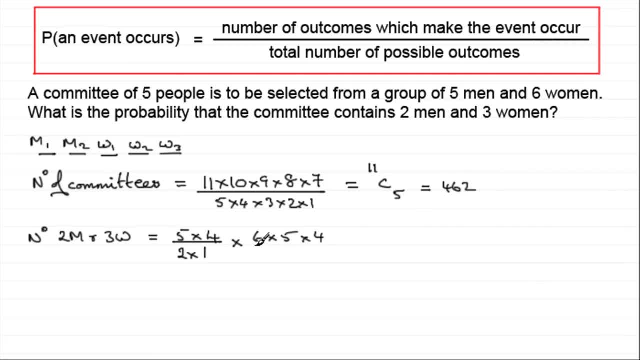 But this would be the number of arrangements of the women. We're not interested in arrangements, just a selection Order doesn't matter. So within these three women, the three women can rearrange themselves amongst themselves three factorial ways: three by two, by one. 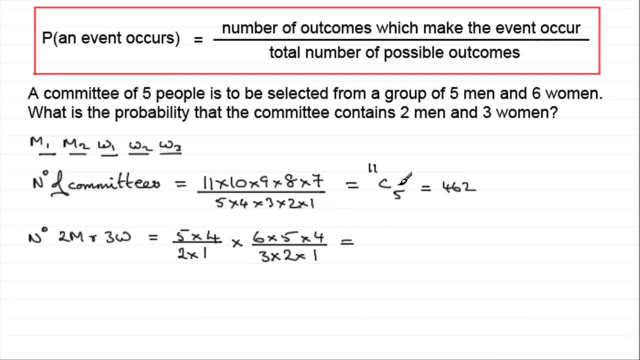 And again, you could have done this through using combinations formally, Because what you could have said for the men is that from five men choose just two, And for the women- we've got six women choose just three. So either way, that's what you could do. 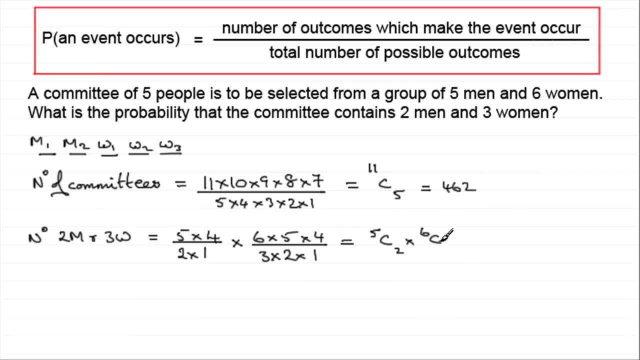 we've got 6 women. choose just 3.. So either way, that's what you could do, And if you work that out, you end up with 10 here times 20.. 10 times 20, giving us 2.. 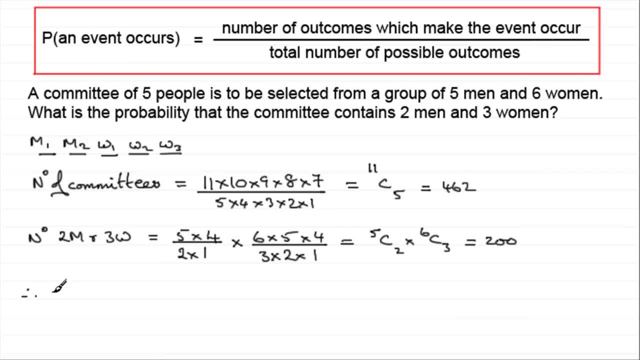 So, when it comes to working out the probability that we have 2 men and 3 women serving on that committee, we use this formula here. So we've got 200 committees, have 2 men and 3 women on out of 462 different selections of committees. 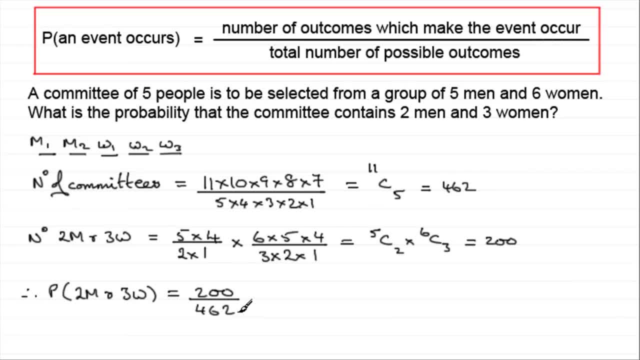 So 200 out of 462.. So 200 out of 462.. You could cancel that down if you like, And that will give us a final answer: 100 over 231.. Okay, well, that's one example using combinations. I've got another example here. 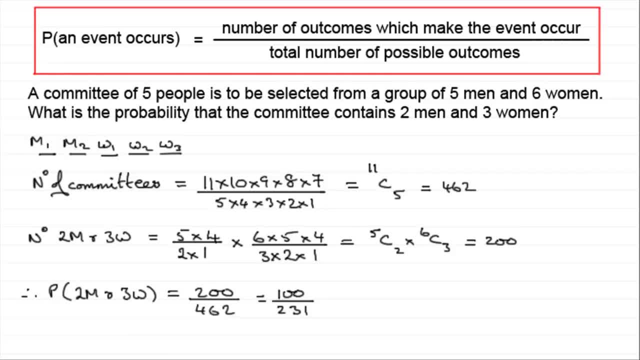 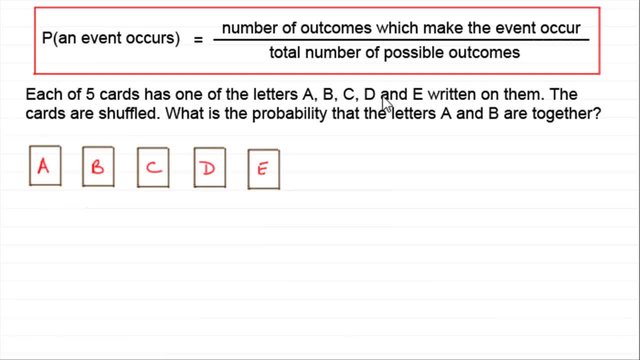 that involves permutations. So in this example, what we've got is: each of 5 cards has one of the letters A, B, C, D and E written on them. The cards are shuffled and what is the probability that the letters A and B are together? 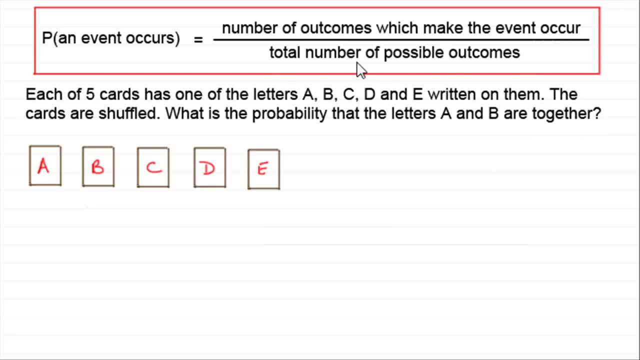 Well, if we consider the total number of possible outcomes, that is, the total number of ways that we can shuffle these cards, what would it be? Well, let's just put an intro here, And that would be the number of different arrangements. 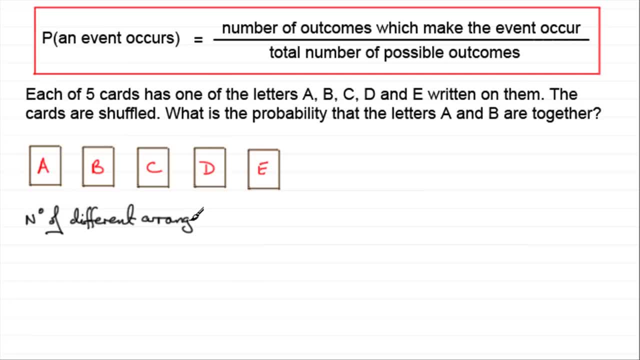 So order does matter here, unlike the previous example. Okay, so we've got 5 different cards, So there's going to be 5 factorial ways of arranging them. 5 factorial comes to 120.. Now we need to look at the number of ways that our 2 cards, A and B, stay together. 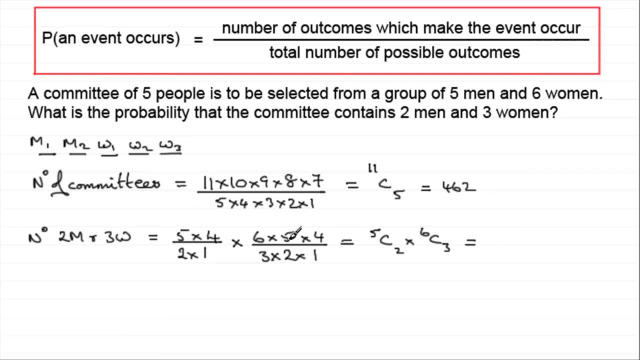 And if you work that out, you end up with ten here times twenty, Ten times twenty, giving us two hundred. So when it comes to Working out the probability that we have two men and three women serving on that committee, We use this formula here. 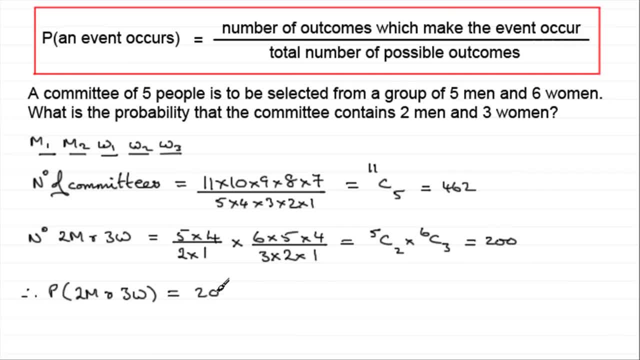 So we've got two hundred committees, have two men and three women on out of four hundred and sixty two different selections of committees, So two hundred out of four hundred and sixty two. You could cancel that down if you like, and that will give us a final answer: a hundred over two hundred and thirty-one. 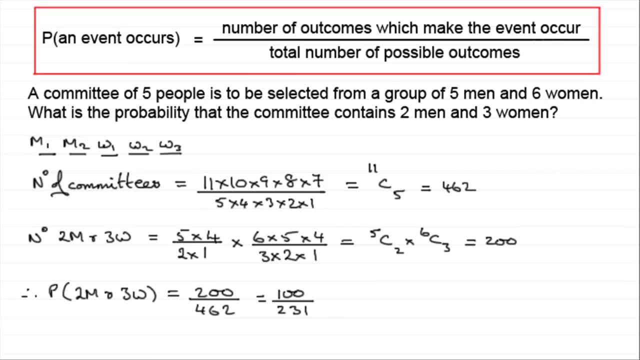 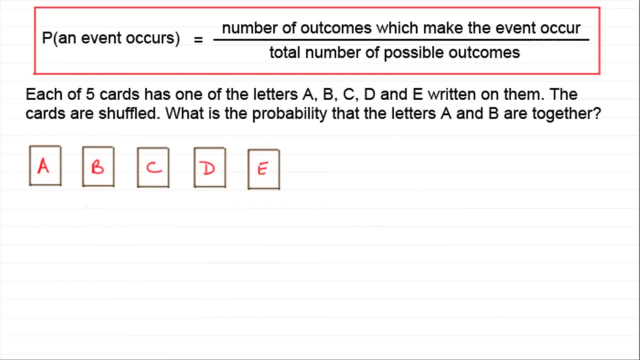 Okay, well, that's one example using combinations. I've got another example here that involves permutations. So in this example, what we've got is each of five cards has one of the letters ABC, D and E written on them. The cards are shuffled and what is the probability that the letters A and B are together? 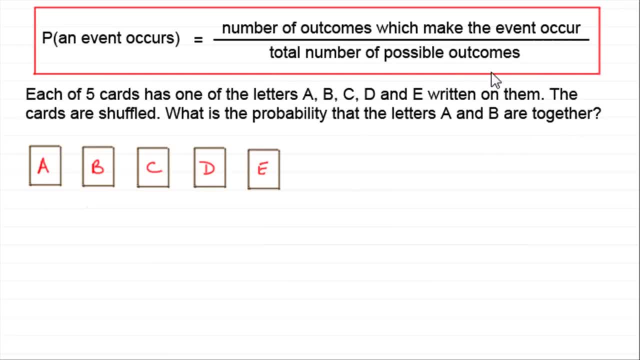 Well, if we consider the total number of possible outcomes, That is, the total number of ways that we can shuffle these cards, What would it be? Well, let's just put an intro here, and that would be the number of different arrangements. So order does matter here, unlike the previous example. 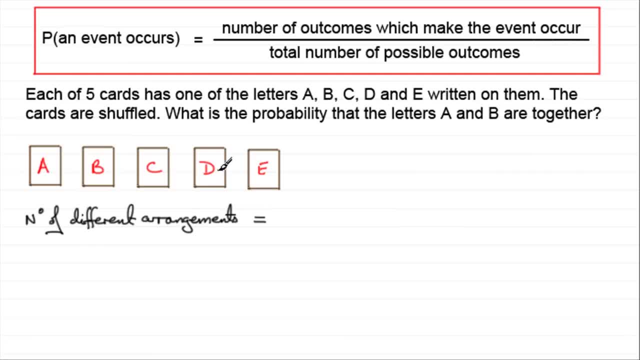 Okay, so we've got five different cards, So there's going to be five factorial ways of arranging them. Five factorial comes to one hundred and twenty. Now we need to look at the number of ways That are. two cards, A and B stay together. 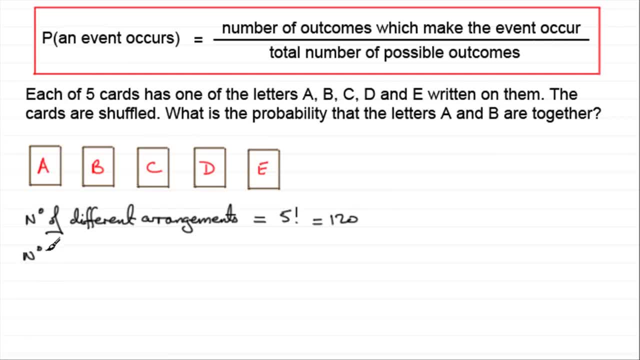 So let's have a look at that number of arrangements where A and B are together. So there's our intro. So with questions like this, remember we parcel them up, Okay, we parcel them up And that's what we're going to do.